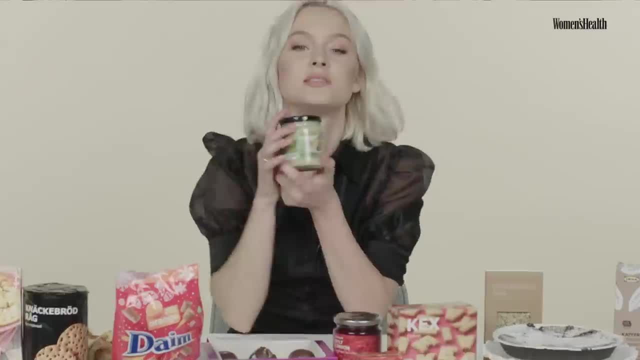 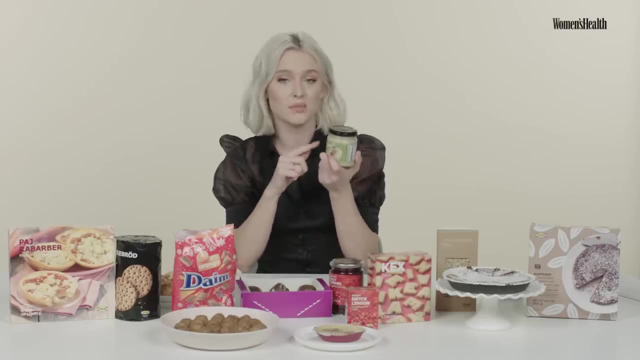 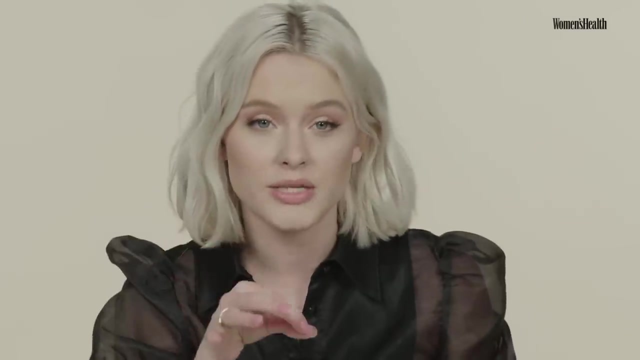 I like the orange. That was nice. Yeah, Seedl, also from Ikea. It's so Swedish. They have these little pickled herring in whatever sauce. This is a mustard sauce. If you want to eat this the real Swedish way, you should have it with small potato, summer potatoes, spring onion, maybe some dill. 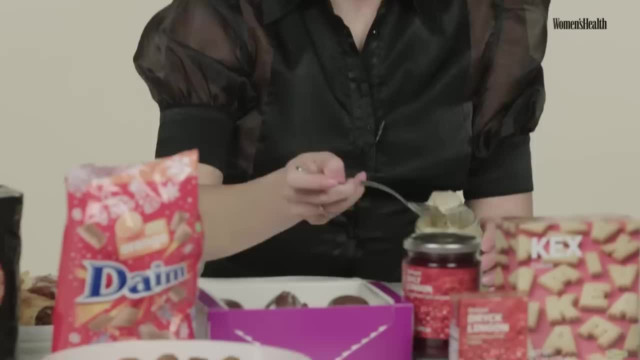 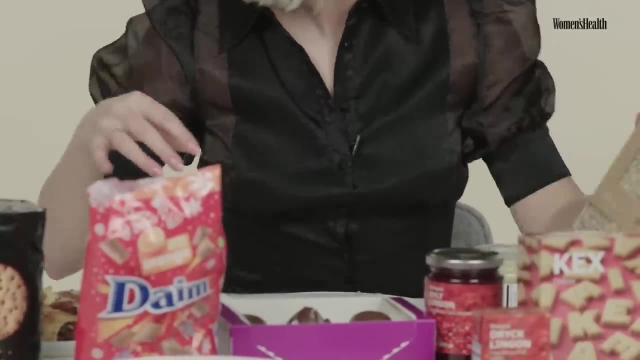 and also sour cream. This is the way to eat it, This is for Easter, this is for midsummer, for everything. And I saw something exciting here too: These ones Kneckebröd. Kneckebröd is like bread, but it's hard. 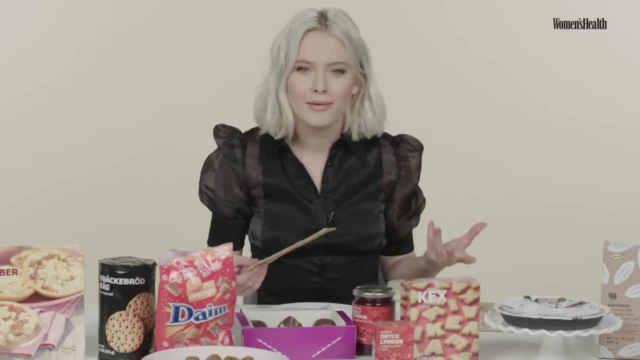 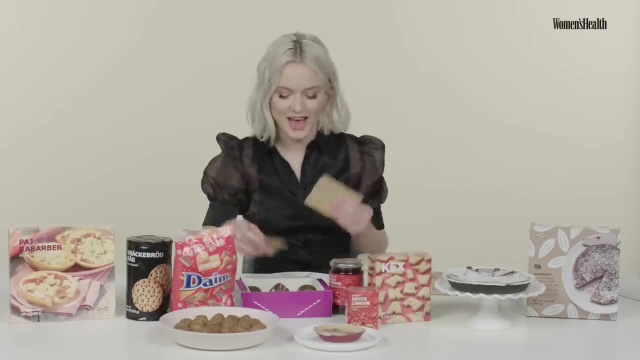 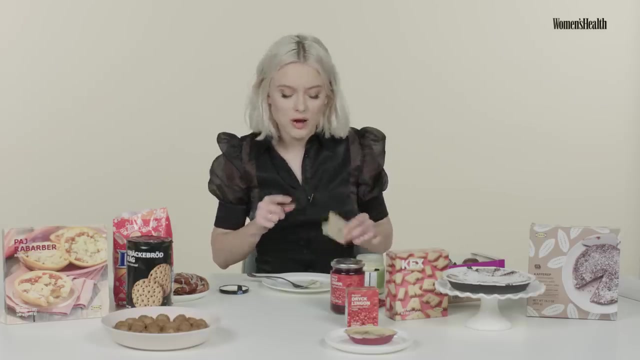 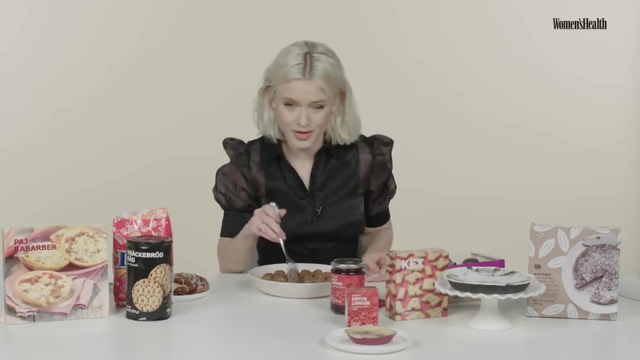 so knäck would be like crack in Swedish. I say so when something cracks like, Yeah, It was really nice with this bread. Last night I had some Italian meatballs and the big difference is the Swedish ones are yummier. Sorry Italians, I'm just being honest. 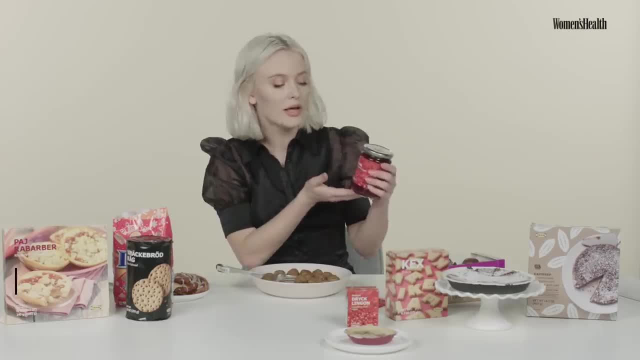 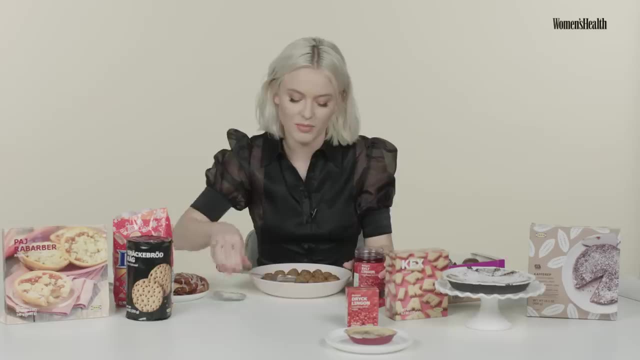 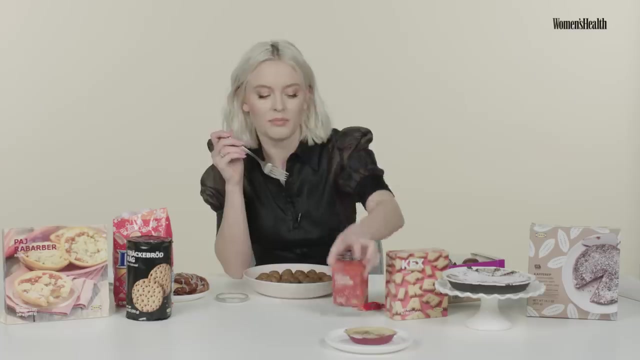 But we can't forget the lingon. Lingon, it's a berry and it lives in the Swedish forest and probably all around the world. And I don't even like this that much. I personally would never buy like a drink, But I do like it a lot on meatballs. 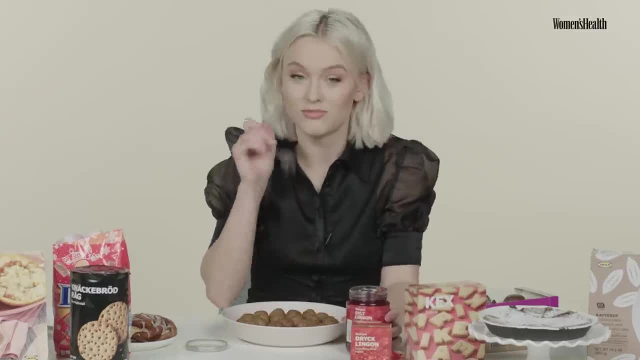 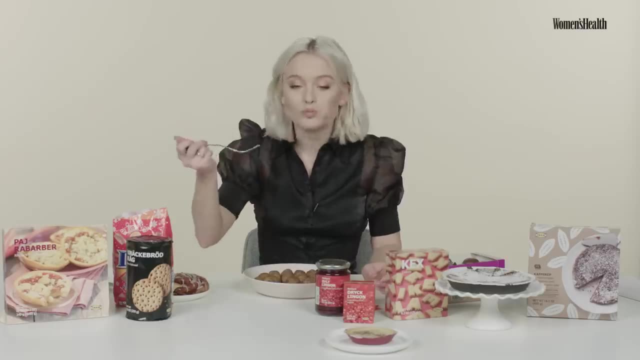 And also if you have pickled cucumber with it, it's really nice. And creamy mashed potatoes and brown sauce. It's how you do it. if you're a real Swede, Very good. What else do we have? Make room for my pie. 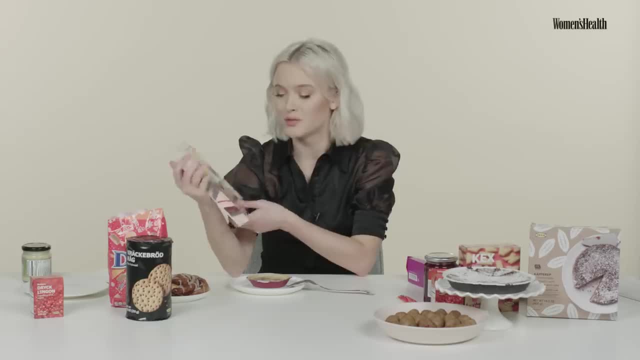 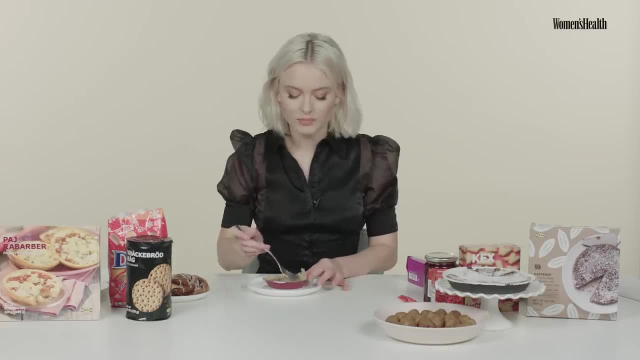 Would I buy it or bear Rhubarbs Really nice. I used to have rhubarbs on my what is it called Yard Garden In my garden, But we have those really big snails that just ate everything. I wish it was a tiny bit more sour. 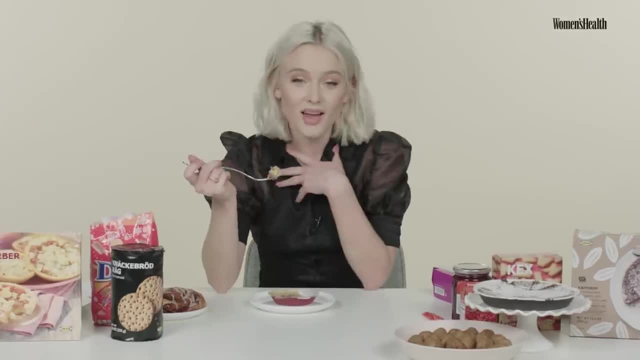 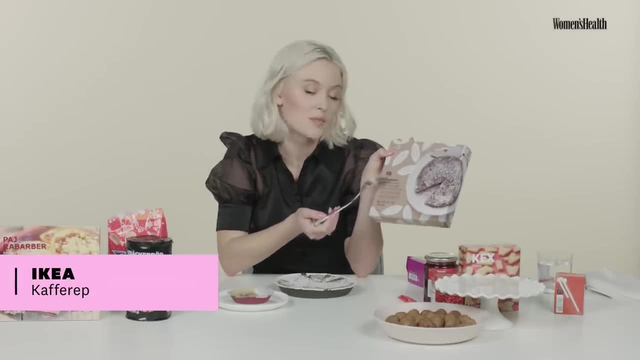 Oh my gosh, I'm like a judge on the Great British Bake Off. I wish it was a bit more sour. Ooh, kaffiria, Kaffiria. it's almost like fika. And you go to this place, which is like a Starbucks.